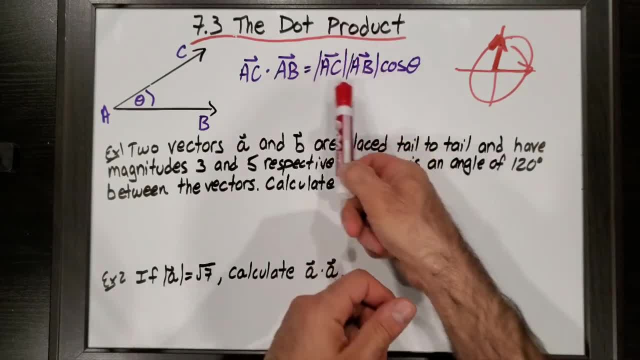 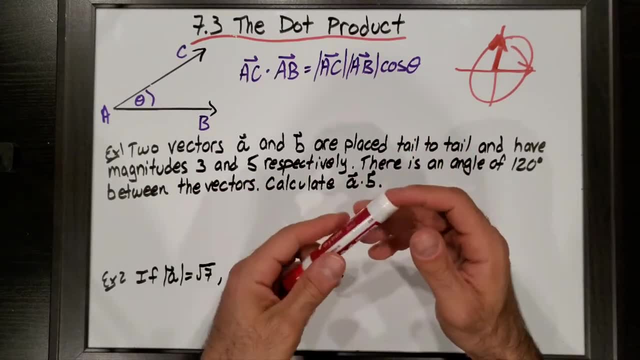 because the horizontal distance in a vertical line is zero. So when this is zero, we know that the dot product is zero, and that's a very useful piece of information because we can find perpendicular vectors by using the dot product being zero. Okay, so it all comes from. 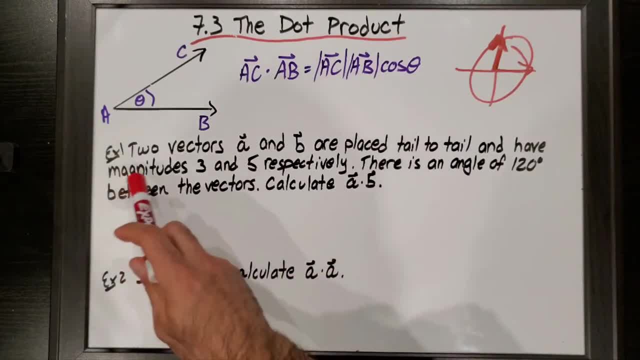 this cos theta right here. So let's take a look at the first example. Two vectors, A and B, are placed tail to tail and have a magnitude of 3 and 5, respectively. There's an angle of 120 between the vectors and we want to calculate A. 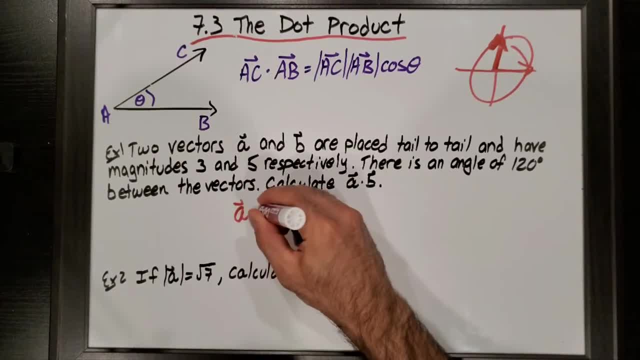 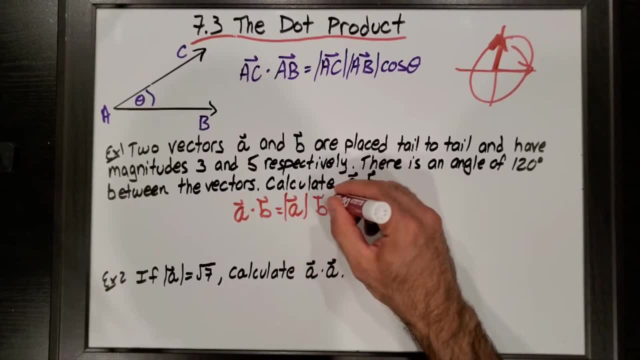 B. So very, very simply, we just use the formula for the dot product that you just learned, and A- B is equal to the magnitude of A times the magnitude of B cos theta. Well, this is just 3 times 5, cos of 120.. So the dot product of A? B is equal to negative. 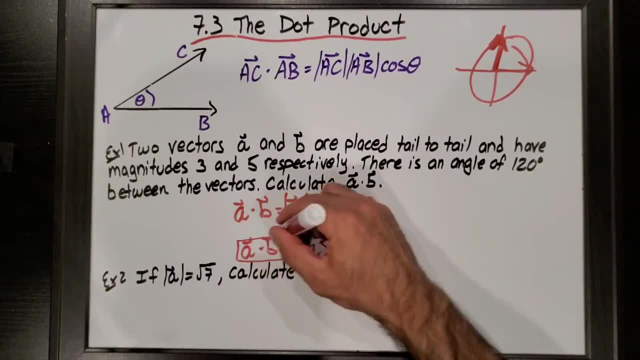 7.5.. That easy If I wanted to calculate the dot product on one vector. so I only know the magnitude of A and that's root 7, and I want to find A dot A. it's the same thing. So A dot A is equal to the. 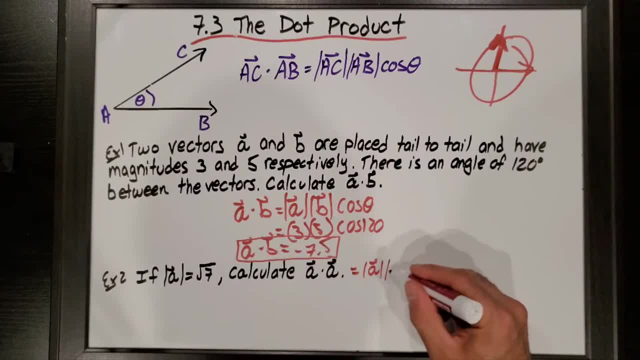 magnitude of A, which we know to be root 7, times the magnitude of A. Actually, no, I don't need cos, because it's the same vector: A dot, A, this is root 7. times root 7, and that's just 7,. okay, You're never going to really see a question like this. 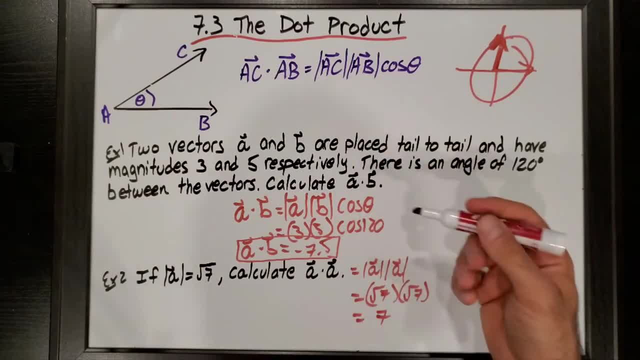 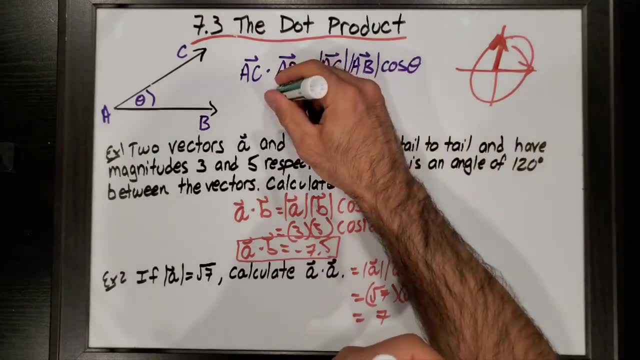 This is just setting up, really a principle that's going to be used for applications of the dot product when we actually change this into a vector, because I didn't really say this, but this right here, this is a scalar product right now. Okay, we don't really have a direction. 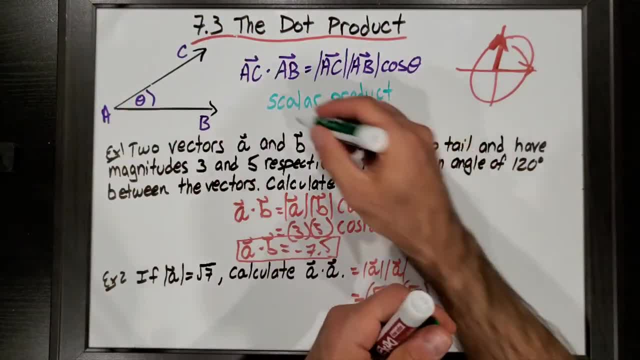 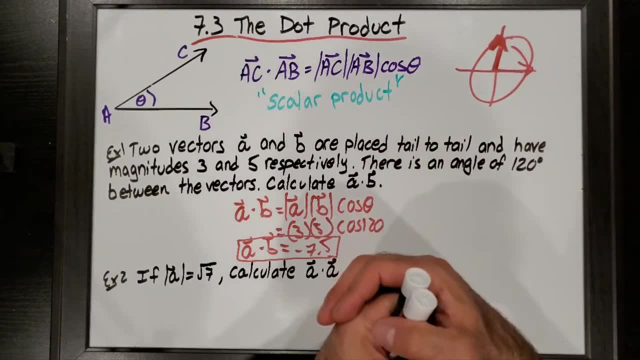 We're just. it could be anything, any magnitudes, any triangles moving around. Right now it's just a scalar product. It will become a vector once we multiply the dot product by a unit vector, and we're going to get into that a little later on. 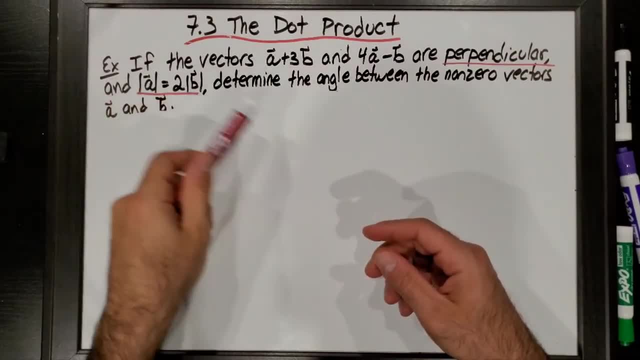 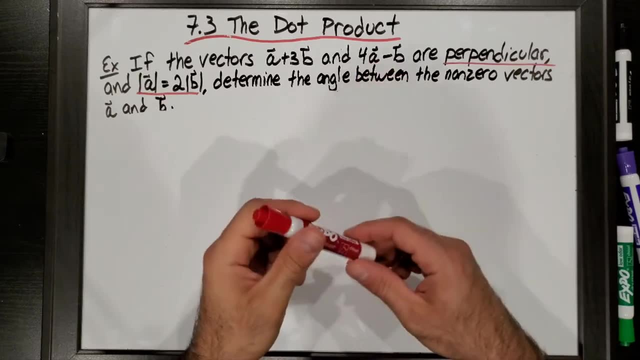 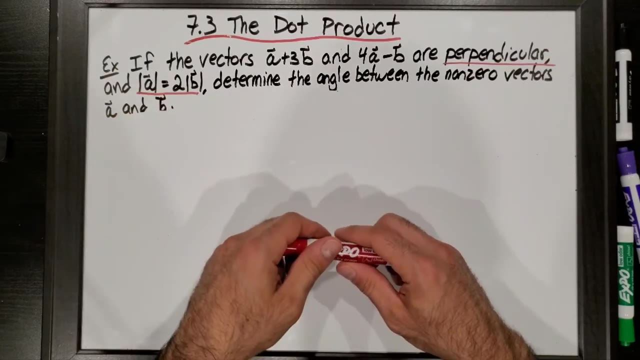 Okay, so for this next example, we have two vectors. One vector is an addition of vector A and B, so A plus 3 of vector B and 4 times vector A minus vector B. These two vectors are perpendicular and I know the magnitude of A is double the magnitude of B Determine the angle. 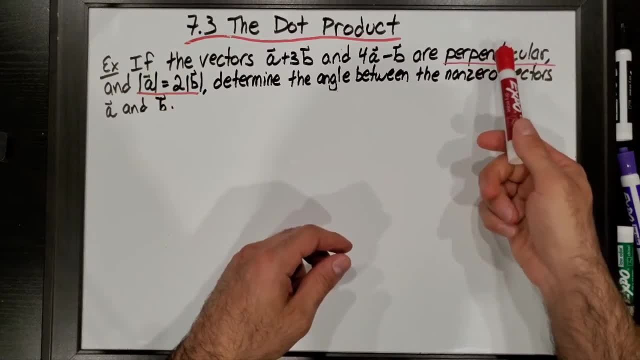 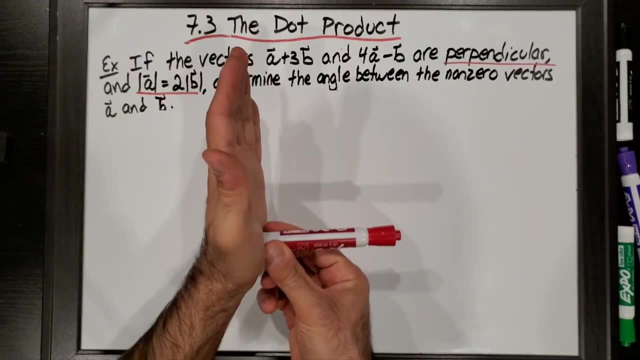 between the non-zero vectors A and B. Okay, so this word perpendicular, like I talked about in a previous little section, we know that if something's perpendicular, the cost of that angle is going to be zero if I find a dot product. So this really helps us start this question. 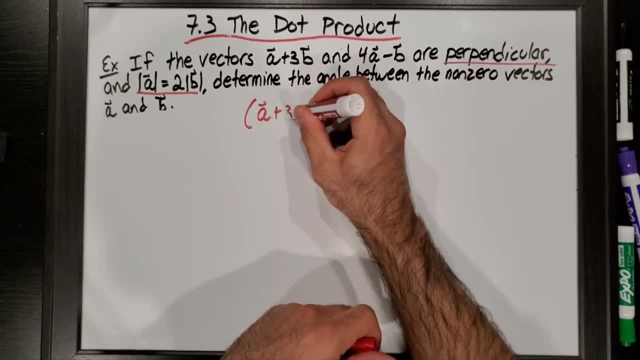 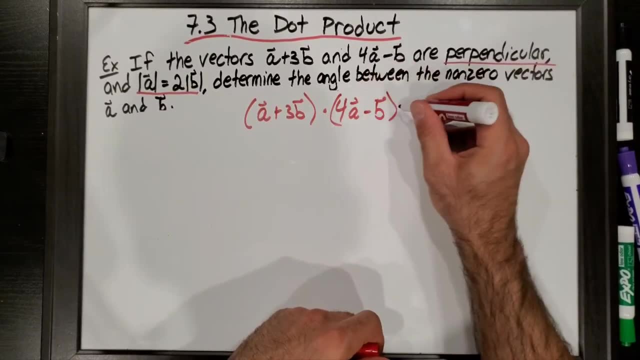 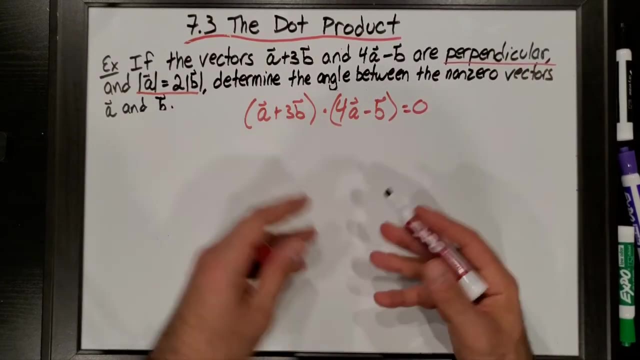 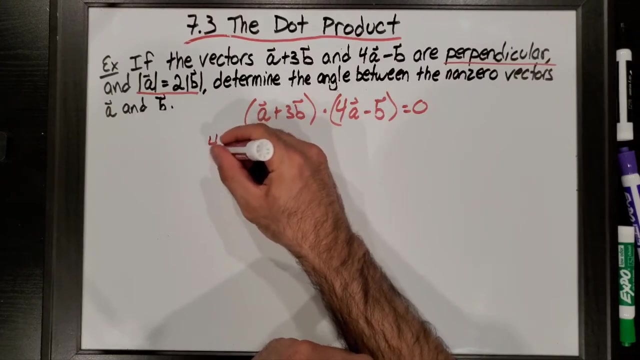 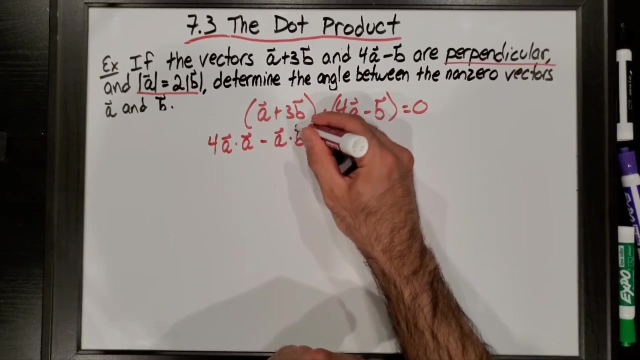 because it tells us that the dot product of these two vectors must be equal to zero. That's it. So I can now expand this, just like you know multiplying binomials, And I can say A times 4A or A dot 4A is 4A, dot A, A dot negative. B is negative. A dot B: 3B times 4A, positive 12,. 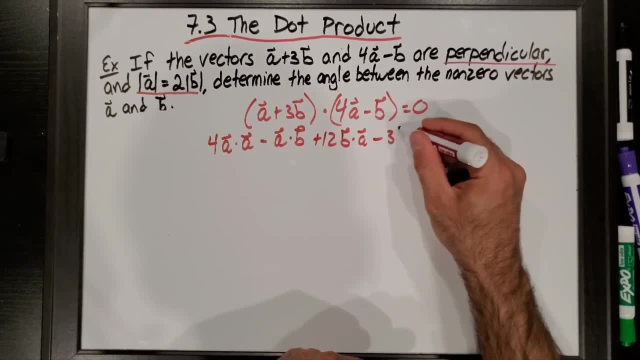 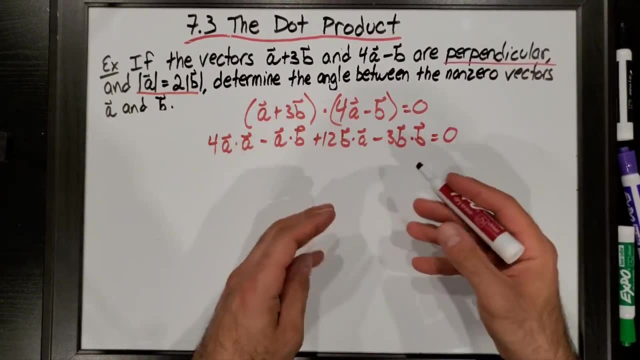 B dot A and negative 3B dot B. Okay, so that previous example, we're going to get into that. So we're going to get into that. So this example with the A dot A, the root 7 times the root 7, that was, you know, the purpose of that. 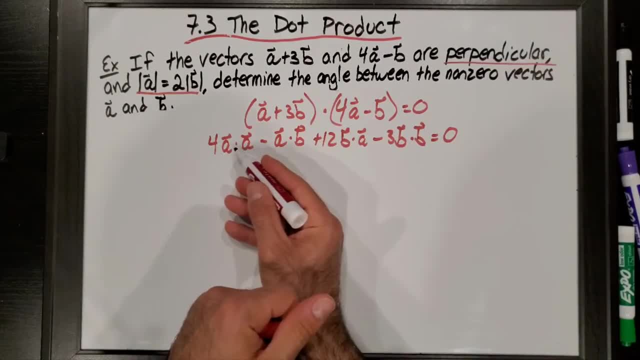 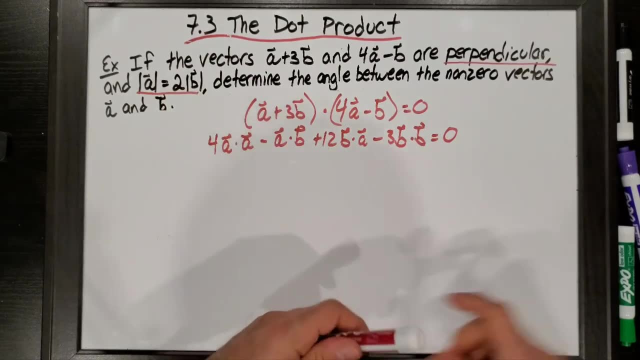 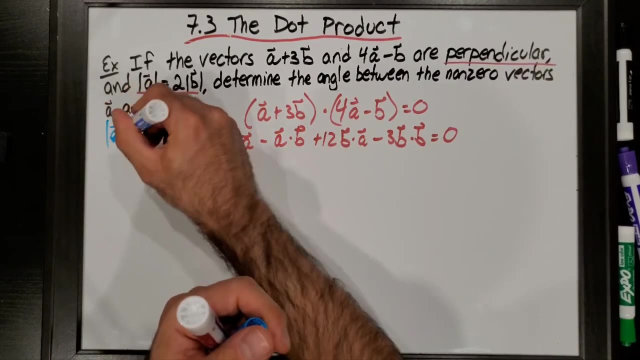 was to show you that when I multiply a vector by itself, using the dot product, I'm just going to get the square of the magnitude, And this is where this comes in handy. If I know that the magnitude of A equals 2B, well then I know that the magnitude of A squared is just 4. 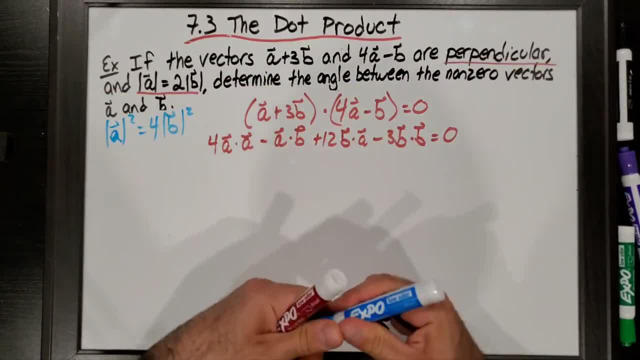 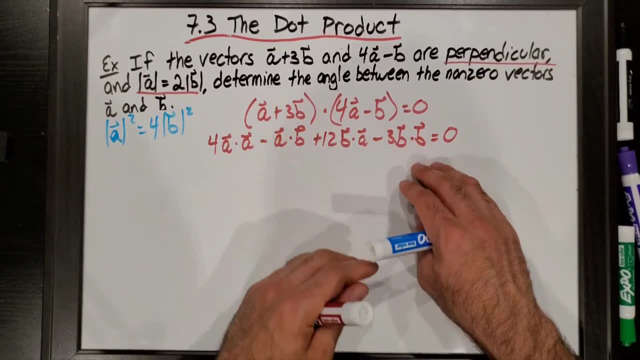 times the magnitude of B squared. So we're going to multiply both sides. And now, anytime I have A dot A, I have a value for that. It's just this. So I can change all of these into variations of vector B. So let's start doing that. 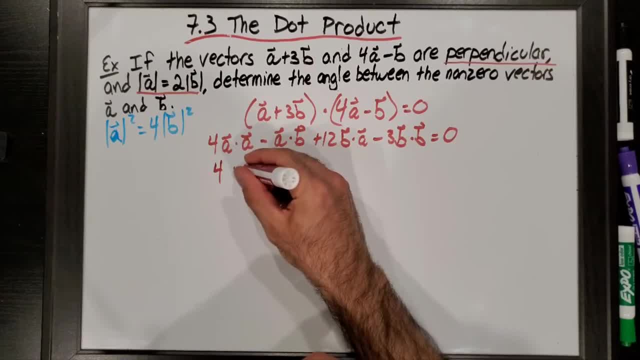 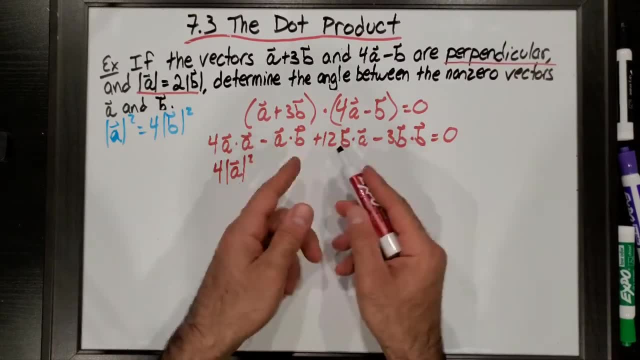 for a second. So this is going to be 4 magnitude of A, squared right In the middle here, A dot B and B dot A, it doesn't matter right, 3 times 4 or 4 times 3 are the same thing. So these are both. 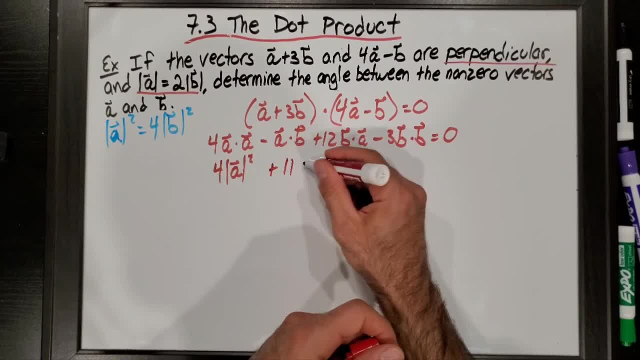 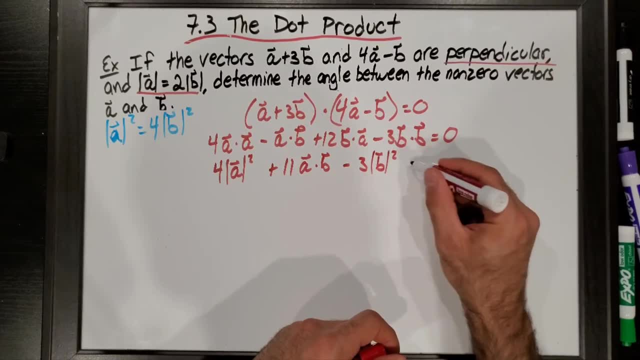 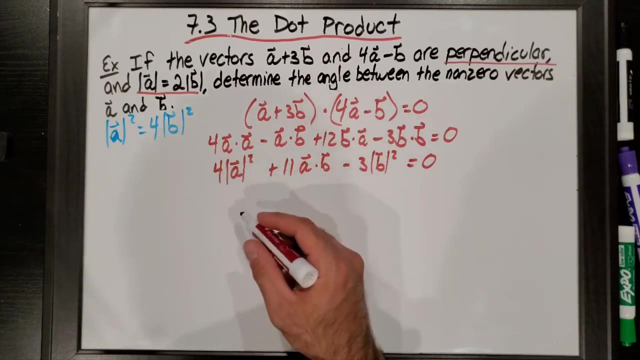 going to combine, because they're like terms to become positive: 11 A dot B- This guy over here is going to become the magnitude of B squared. OK, So now I can actually replace A- the magnitude of A squared- with its value. 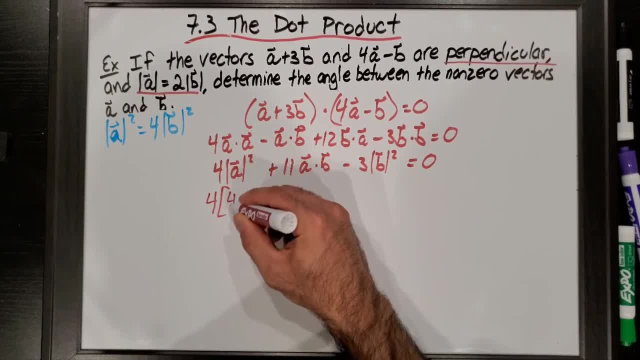 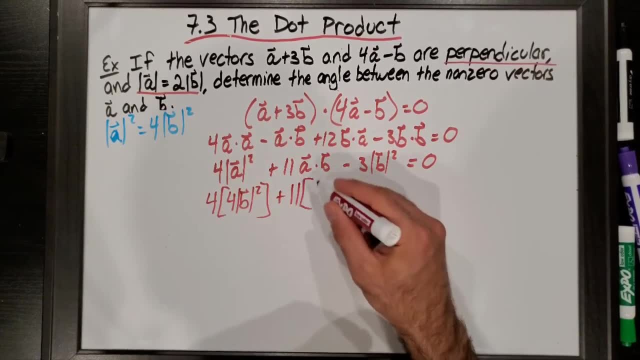 in terms of B. So this is just going to be 4 times 4 magnitude of B squared, plus 11 A dot B. Well, A dot B is the magnitude of A times the magnitude of B squared. So we another have the same thing over here. We just are going to get this piece here. So we also have, for example, a plus B, And then when we do that, we also have a bigger ratio of B. each time we multiply two and 5 times 2.. So if you look at that side, we just have 4 times the magnitude of A squared by thegos vorneut. 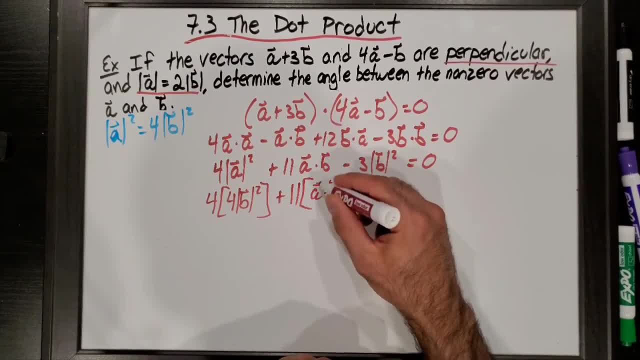 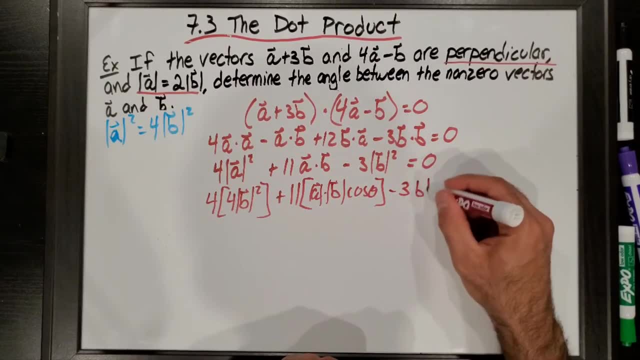 The magnitude of A squared. Now, when I flip over this, we have 4 into the other side, times the magnitude of B, cos theta minus 3, magnitude of B squared, and this all equals 0.. Okay, so I can just, you know, simplify some things here, make a 16 here. 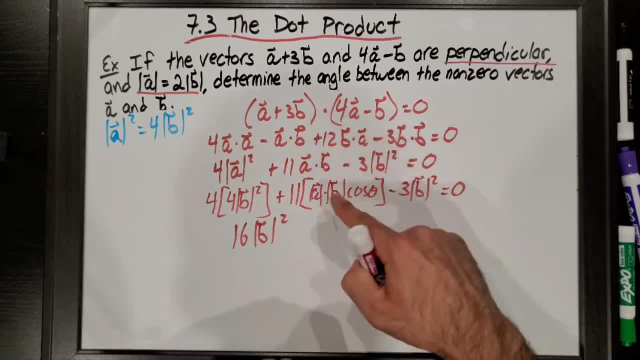 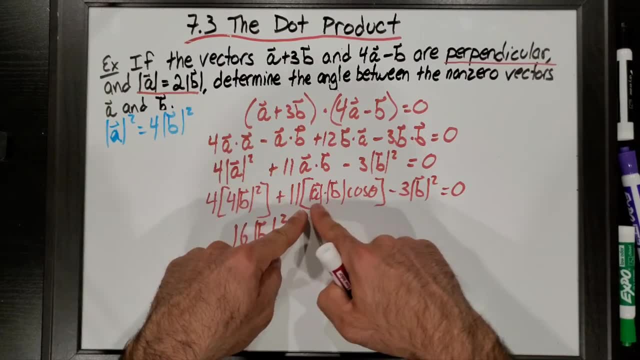 Sorry, I was supposed to put the magnitude, so the magnitude of A, in here. I'm actually going to replace it because I don't want to write another line, but the magnitude of A is just going to be 2B, so I'm going to have a 2B squared in here. 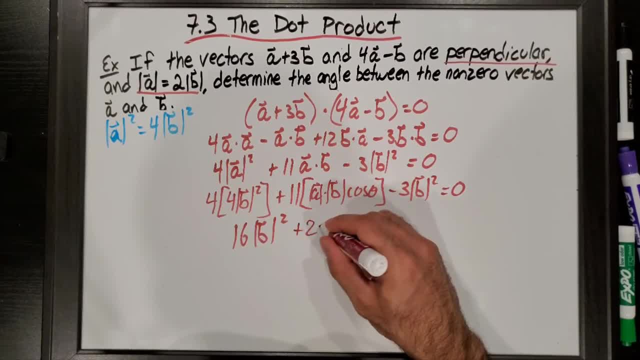 if you see that happening. so this is going to be a plus 22,. magnitude of B squared cos theta. so I'm going to go over that one more time. This A, right here. I'm going to replace it with the value of A. 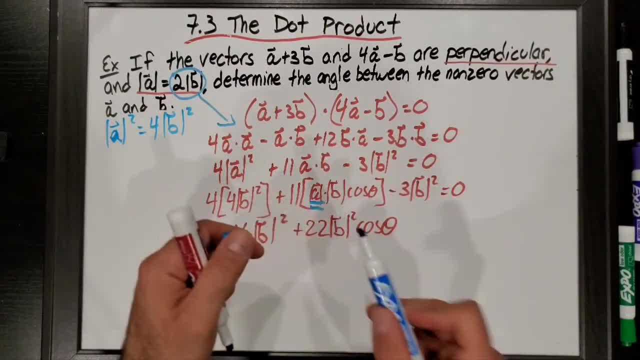 Okay, so it's just 2B. and now I'm going to have that magnitude of B squared and I'm going to go over that one more time. Okay, so I'm going to go over that one more time. I'm going to call it the magnitude of B squared. 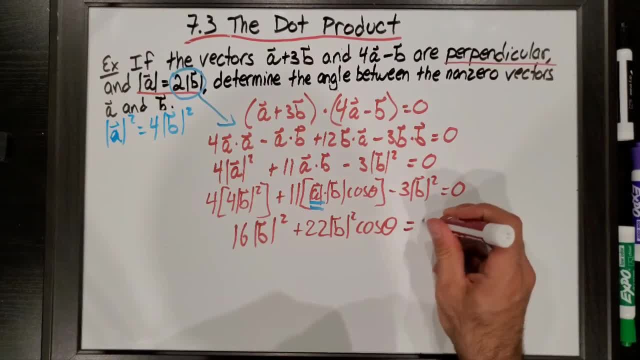 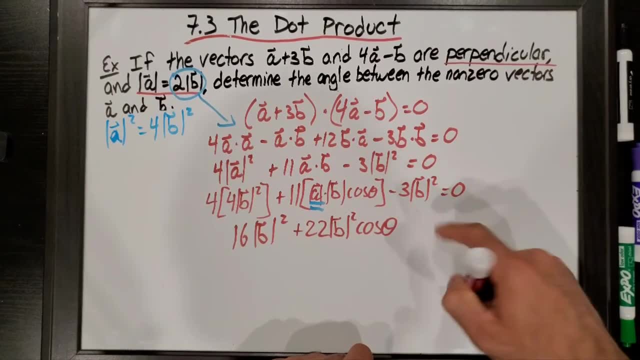 Okay, and that 2 combines with the 11, make it a 22, and this is equal to 0.. Okay, so I'm almost there. Oh, I forgot the minus 3.. How dare I? Minus 3, magnitude of B squared. 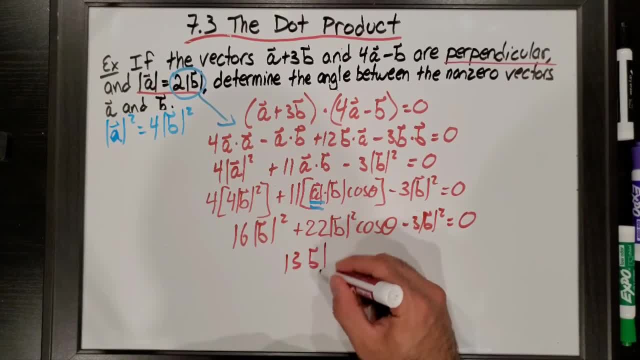 So these guys are the same. I can combine them. This is going to be 13B squared plus 22B squared, cos theta equal to 0.. And I'm slowly solving for Or cos theta here, right, So I can say: cos theta equals negative 13B squared over 22B. 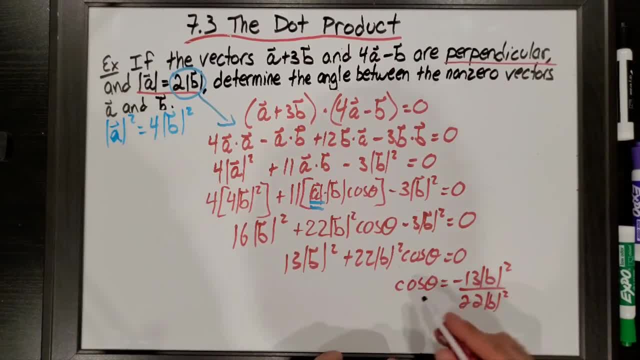 B squared. sorry, The B squareds cancel out. So I'm just finding the second function of cos, or the inverse of cos of negative 13 over 22, because the B squareds cancel out. So theta equals cos negative.